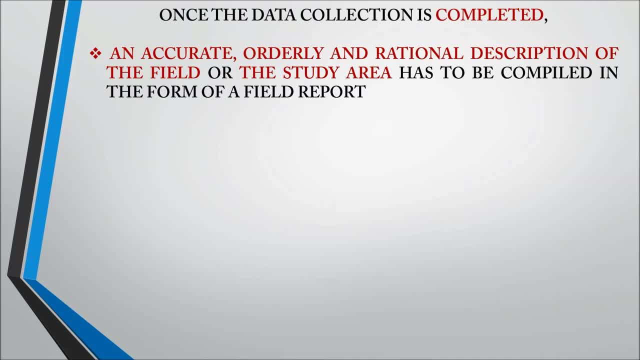 Now, orderliness means a scaling is involved, a sequence is involved, a pattern is involved, right, That's why order is important And rationality is with the least bias as it can be. So biasness has no scope when we are talking about a basic idea of field research and a report writing. So accurate, orderly and rational: Remember these three key words whenever you are making a field report right. 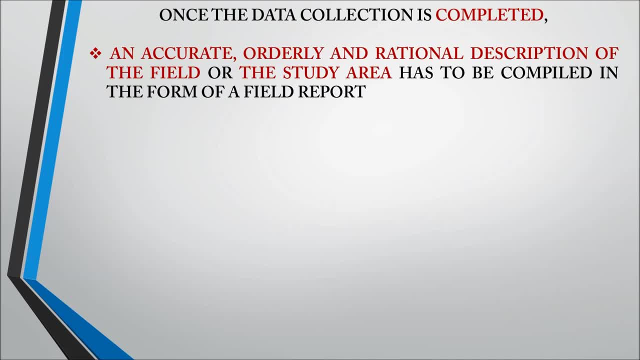 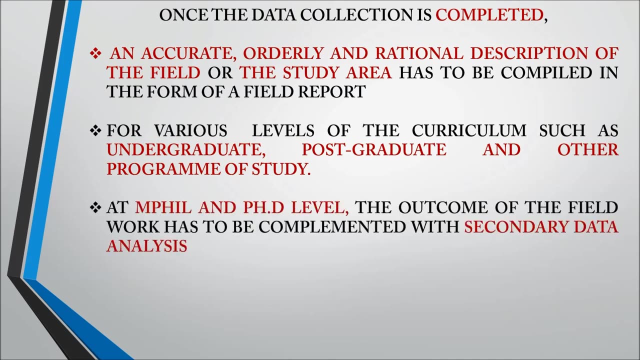 So for various levels of the curriculum, such as undergraduate, postgraduate and other program of studies like MPhil and PhDs, this is applicable, that it has to be accurate, Accurate, orderly and rational in nature. So at MPhil and PhD level, the outcome of the fieldwork has to be complemented with secondary data as well. 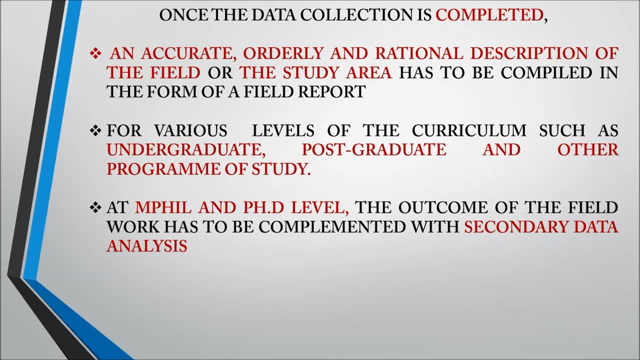 But undergraduate level. if it is just a field report, then maximum of the primary data has to be included, apart from some secondary sources, Alright. So the focus has to be at undergraduate level on the primary surveys, but in MPhil and PhDs it has to be a balance among the two. 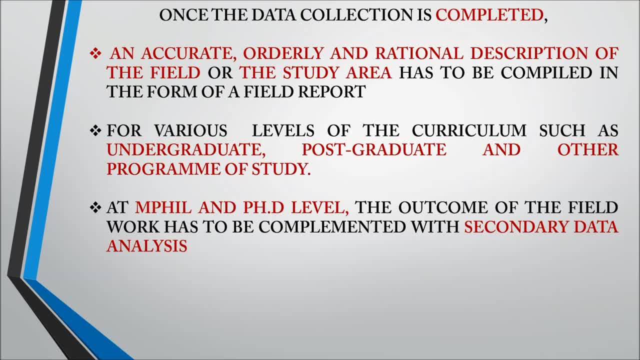 So secondary data as well as the primary data collection. this is all based on the primary data In a firm full. make sure all dataoperation is automated. Okay, now see this scene of work in- prepares everything in a mess. diligęza has to know, But in MPhil and PhD need to keep everything in order. 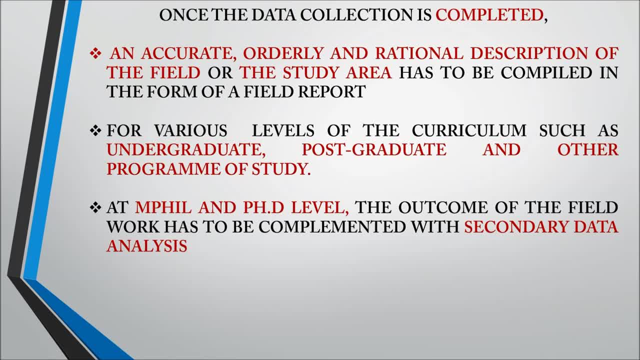 So secondary data as well as the first two other tasks to be done that need to be carried out at the end of the assessment data collected from the field has to be balanced in an order, right. so final dissertation or thesis, which has to be submitted after fulfilling the various 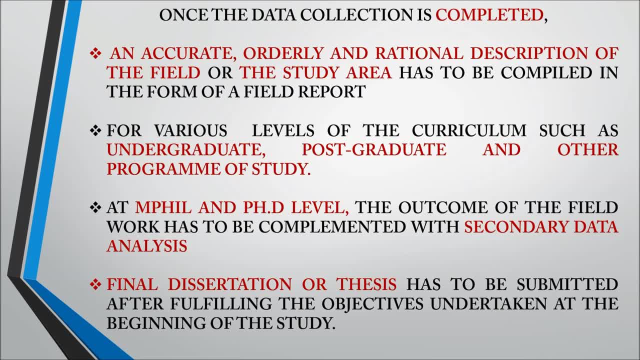 objectives that we have taken in the beginning, doesn't it? a research starts with the idea, the objective of what has to be done. so at the end, when we are submitting the report, the dissertation of the thesis, has to be clearly stated that it has fulfilled the objectives undertaken at the beginning of the 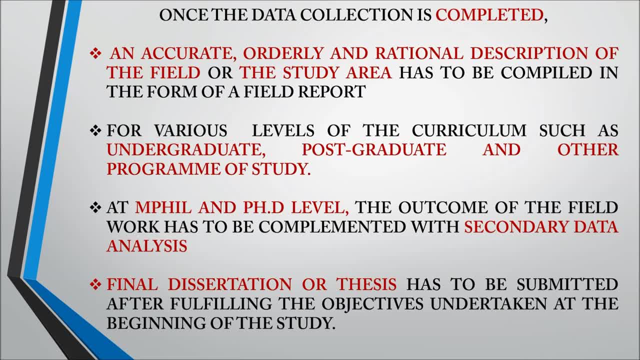 study. so this is the basic idea of writing a report. so whenever we start writing, we must have this concepts and idea about how to write a report. but before that, what is the basic ingredient of writing a report? what is the basic idea behind it? isn't it now so according to the methodology of field report? 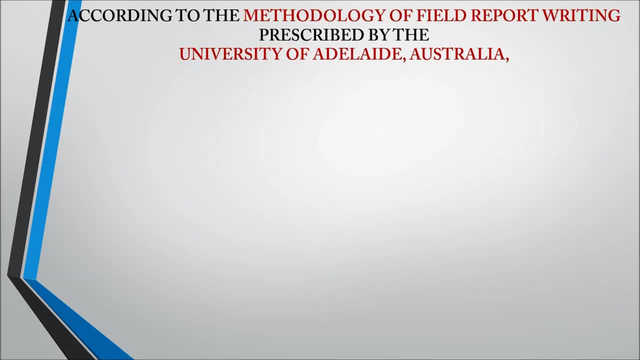 writing. let's take a reference from University of Adelaide, Australia, a standard reference, that what is the methodology? talking about field report writing, right? so in producing a field report, the researcher or the student normally addresses following questions: so what happens? the field report must address, must answer these questions. the first question is: what did you do the first? 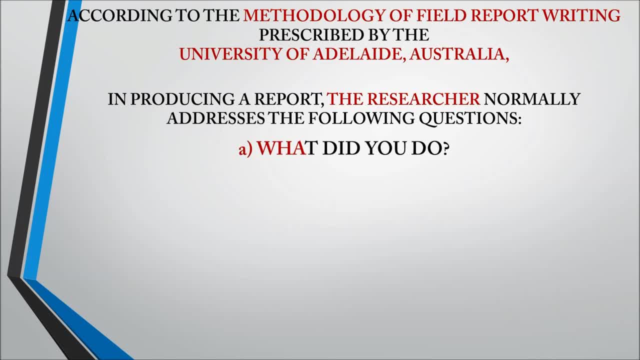 question is: what question? what exactly did you do what? what was the study undertaken then? what question is further added by? why question? so? why did you do it? what was the purpose? why there was a need. so you have to establish that need when you are writing the. 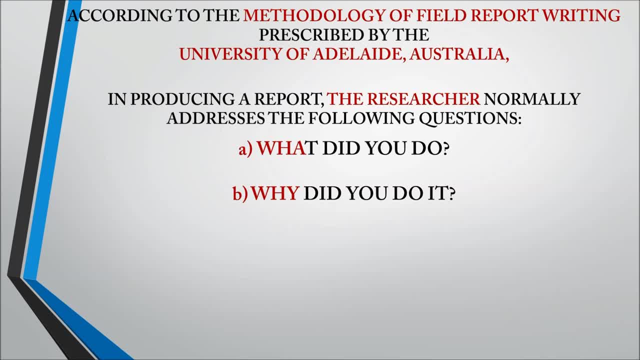 report ultimately, isn't it? then? how did you do it? this is talking about the research methodology that we discussed, isn't it so? what was the data, how was it collected, what were the methodologies involved and what were why that particular method was applied for data collection? isn't it so all? 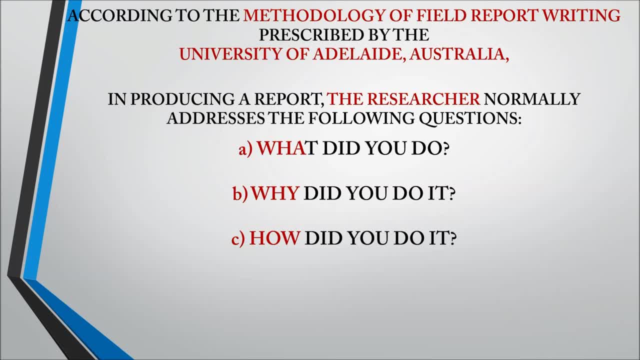 those things comes under how you did that work- fieldwork, isn't it? then what did you find out? it means now we are talking about the results, the analysis of the data that we collected. what was the result all about? okay, so what are the finding and what does the findings mean? so findings have nothing to do just with the results. that 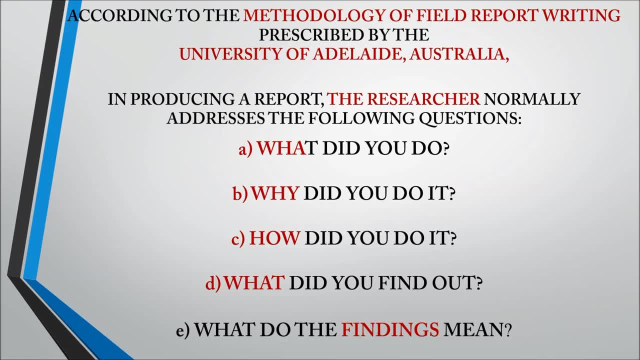 you derive. just remember, the research doesn't end on just the result that you derive from data analysis. first there that result has to be interpreted. it means we have to interpret the results in the context of the study, in the context of the study area. because if we just put the analysis results, 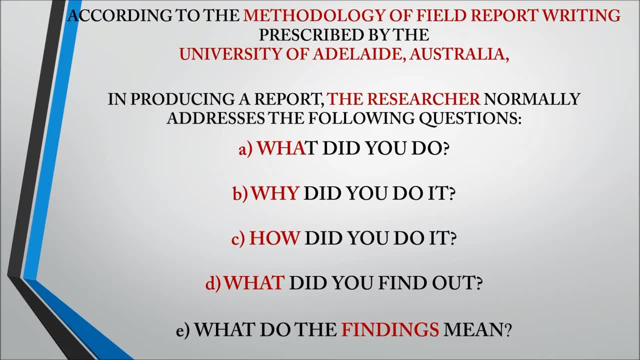 in statistical format or just the result of the data that we analyzed, it has no meaning. we, as a researcher, have to give meanings to our findings in the context of the study. so do not stop just after analyzing a data. the result of the data has to be finally interpreted. that's what the 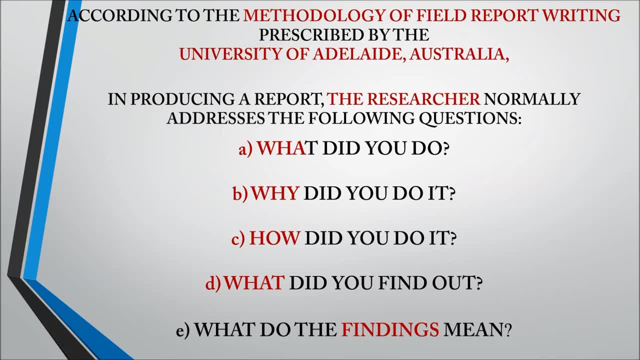 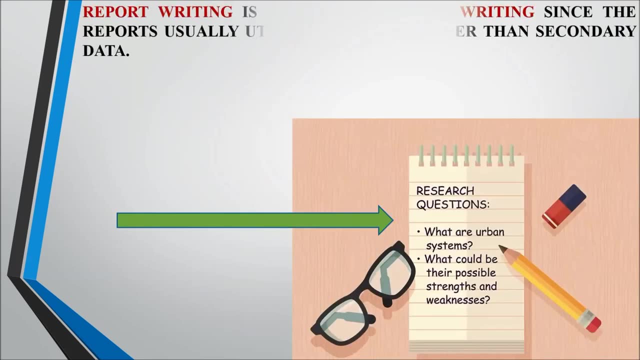 last and the fifth point is: so this is the entire methodology of writing a field report. so whenever you are writing a field report, remember to answer these five questions. okay now, so the first basic thing about report writing is that it is different from an essay writing, so do not confuse or do not. 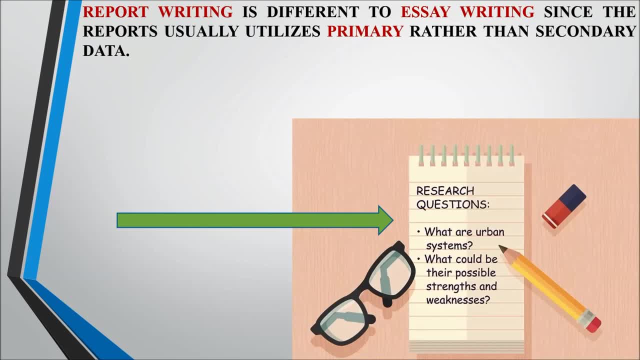 make that same way that essay writing you're doing. right, because I said writing is different. the reports normally utilize these primary surveys, primary data, then security data, right? so that is most important difference. then they are formally structured, so a report is not just random writing. okay, it has to be a structured format. so formally structured and 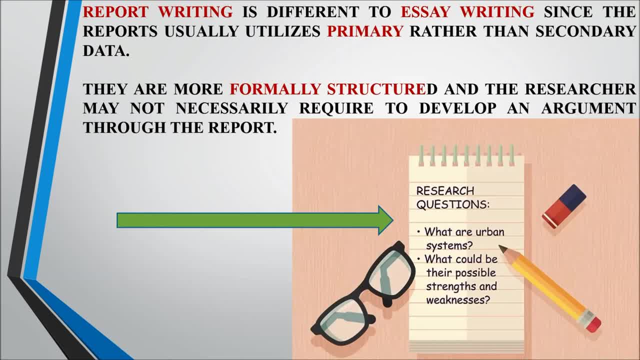 the researcher may not necessarily require to develop an argument throughout the report. it's not necessary that you apply argument in every section, because it's a formal structure, so every section has its own importance, and then you have to compile it and remember that addressing the research questions is the main purpose. so what were your research questions in the beginning? 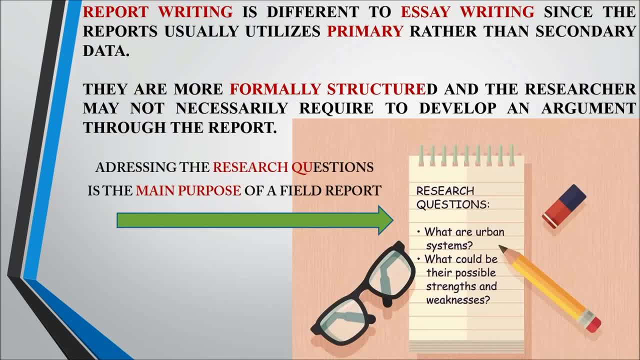 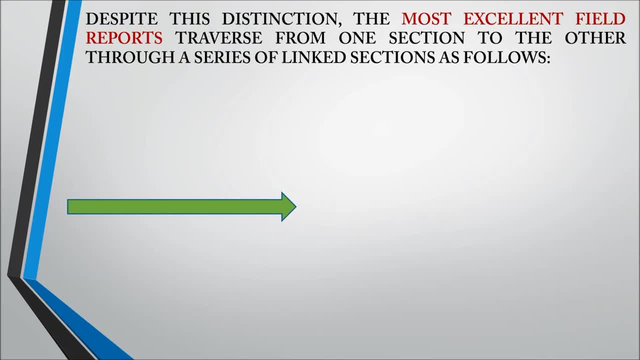 that is the main purpose of the study. all right, so despite this distinction, it's important that most excellent field work field reports traverse from the first to the end sections in a linked manner in this particular way. so let's look at that. so introduction is the basic idea, right, introduction to your research, where you discuss about the details, about the 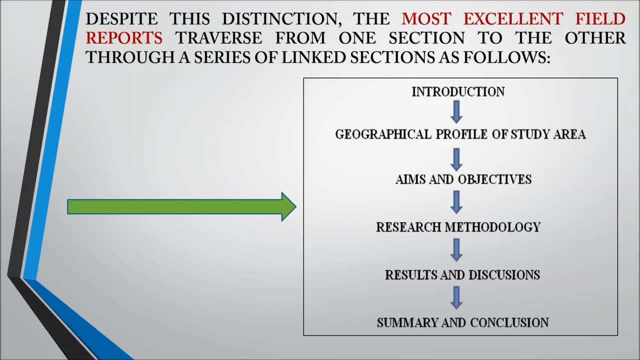 conceptual part of it and research questions, then you're talking about the area of research. so geographical profile you must address. if you are talking about a particular area where you're going to do the fieldwork, isn't it then aims and objectives? so if you're doing your aims, 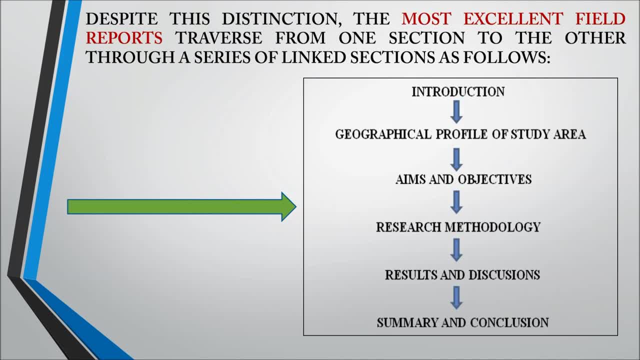 and objectives. that it means. then you are fixing your work, your goal, then you are applying the research methodology- completeness, you are discussing it and then you are applying it, and then you're deriving results and discussions and then, finally, you're writing the summary and conclusion. so this is a basic structure, but remember, the basic structure has to be provided. 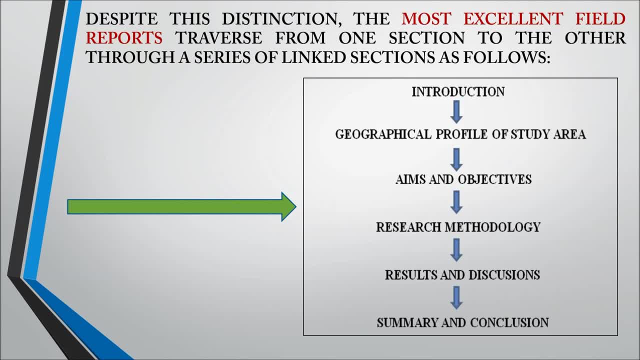 with certain in-between points. for example, in-between points like geographical profile of study area will have to have the entire physical and human geography in the context of the study, isn't it? but before aims and objectives we also must go through all the literature that is available. so 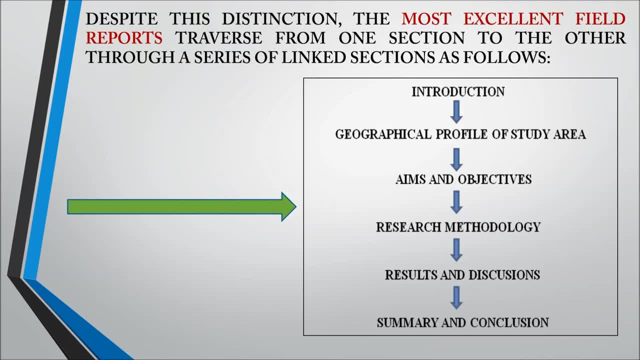 then you must consult all the literature that is available, isn't it? otherwise how will you fix your aims and objectives? so that is in between. but this is the basic, excellent structure that you can think of writing any basic field report right, and you can further improvise. that will see that how you. 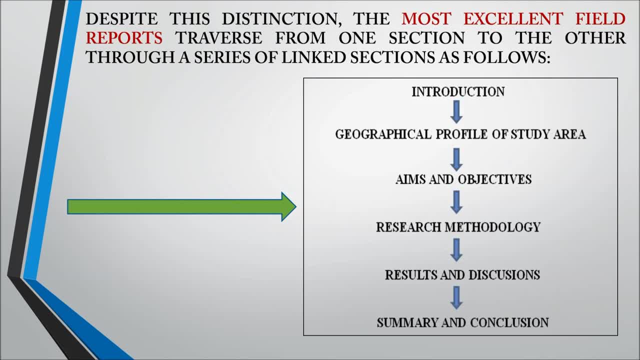 can improvise upon this basic structure. so this basic structure has to be improvised further. so, basic introduction, study area, aims and objectives, research methodology, results, discussions and summary. this is a basic structure and then you must consult all the literature that is available. you have to build your building on this basic structure of the report. okay, so you have to add you. 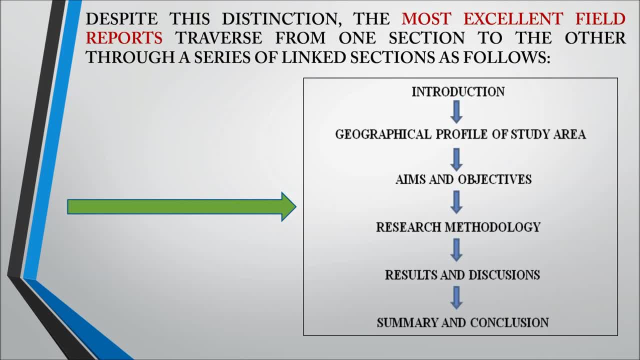 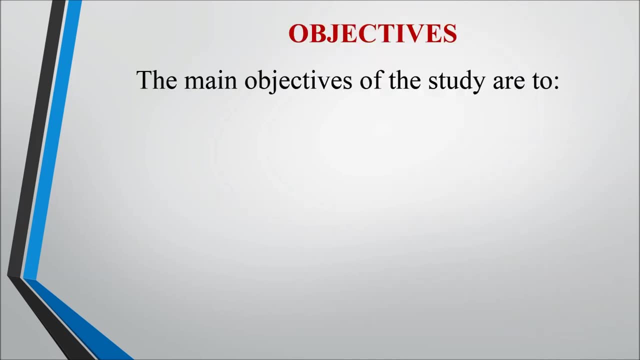 have to change the title, subtitles. you can do whatever you want on this basic structure. so remember this basic structure, which is important here. okay, now objectives. so objectives are important because you must mention it in a given priority, in a format. so how to write your objectives? so i'll tell you a simple way to understand how an objective is written, so you 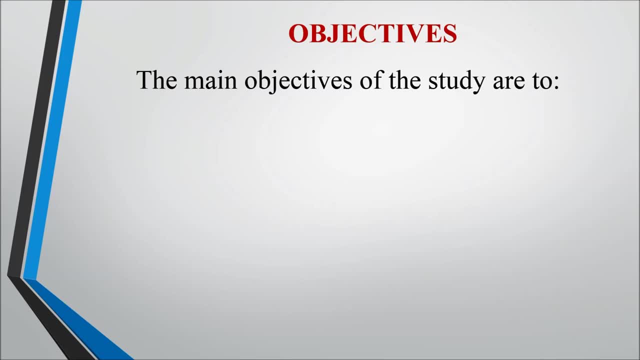 we have a study and its main objectives have to be listed, so it has to be listed in this particular way. for example, the first objective has to be regarding the identification, the what question. remember the questions: so what, how, why? so the first question is: what so? the identification of 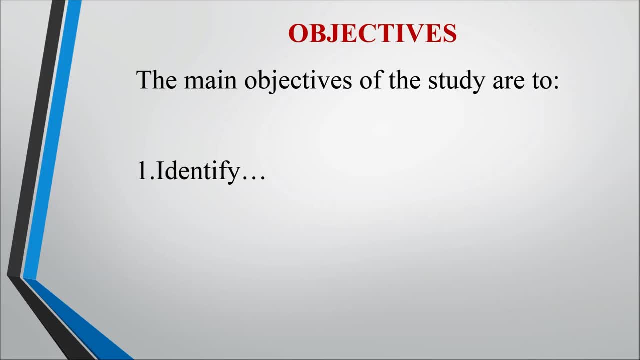 the study context is important. identification of the research problem is important. so first objective has to start from the identification. so what you can write is: the objectives of the study are to identify such and such problem in a given area. right, then the second can be assessment. now comes the how and why wall apart, remember. so identification, then assessment. 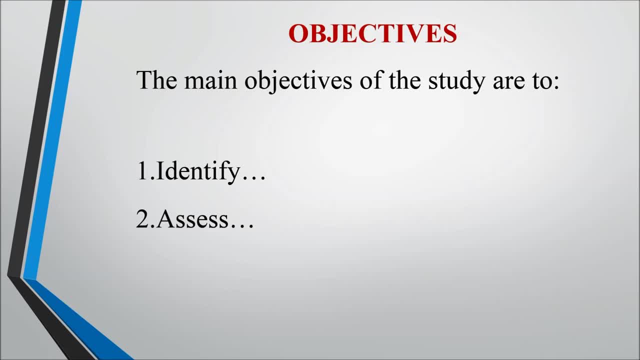 so to identify, then to assess such and such problem, then to analyze. so third is the last section of analysis of what you're assessing. so assessment is you're going to the field, collecting data in a particular method, you're applying and then you're bringing back and 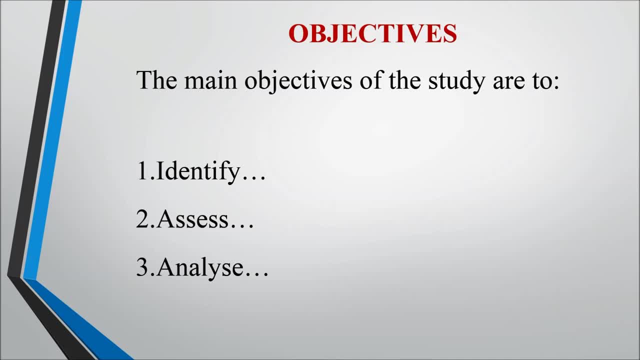 then you're analyzing it, isn't it? so third step is analysis and fourth step is formulation of different strategies, suggestions, on the basis of the first three steps. so this is a sequence that you need to follow, and if you don't find any other word, you can use this method to prepare any. 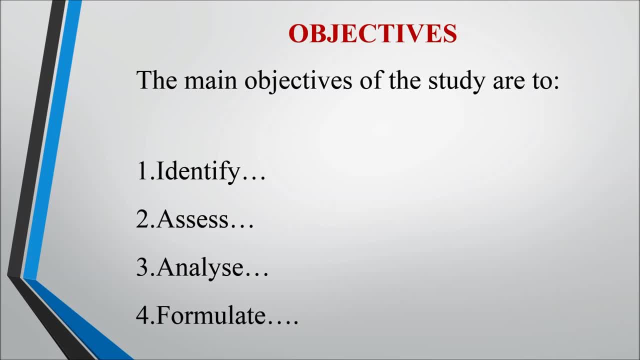 research proposal in terms of your mphil or your phd or any research proposal at any level. the basic objectives can always be listed in this manner. the manner of analysis is to identify such and such problem, to assess such and such problem, to analyze such and such problem and to formulate strategies based on the identification, assessment and analysis. 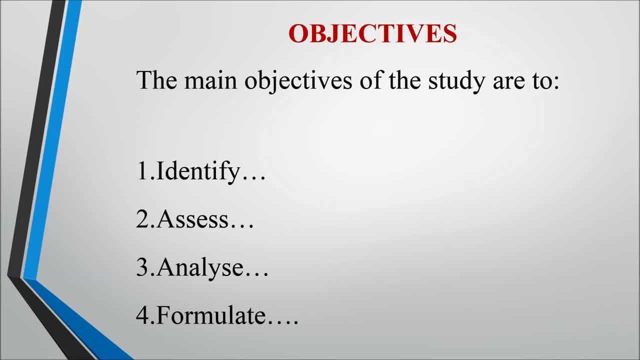 isn't it? so this is how we state our objectives while writing a report. remember to write your report with a focus on these keywords of the objectives. so your objectives must have this identification, assessment, analysis and formulation. words, for that matter, even if they are not words: it. 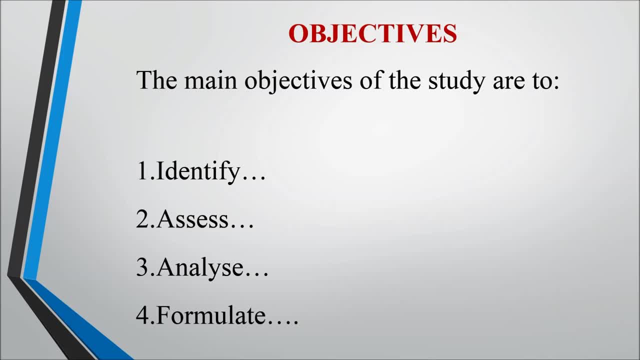 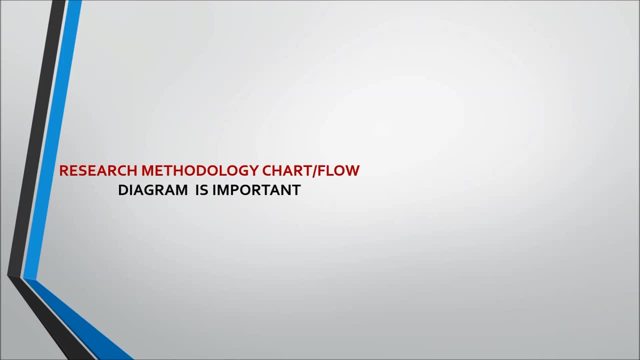 must be part of your objectives. all right now. research methodology chart, or a flow diagram, is one of the most important aspects when we are writing a report. finally, why? because for a reader, a neutral person, who doesn't know what you're doing, what you have done in your work, this one chart can summarize it for him, that what 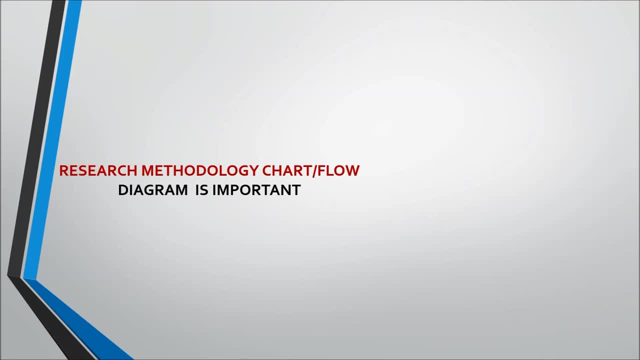 is the flow of your work, so you have to represent it in a very clearly stated manner, in a flow, in a flow diagram, in a flow chart, isn't it? for example? this is example for of a flow chart, so it is one of the examples you can design your own. so a research methodology will have primary data and 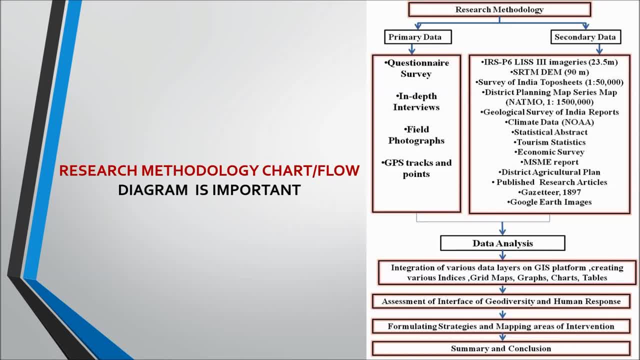 secondary data, which will be clearly defined in terms of what are the ingredients of your primary data, where are you collecting it from? and then secondary data sources. then how are you analyzing it? and then how are you proceeding further till summary and conclusion. so this is the basic idea of a flow diagram that is important when we are writing it. finally, 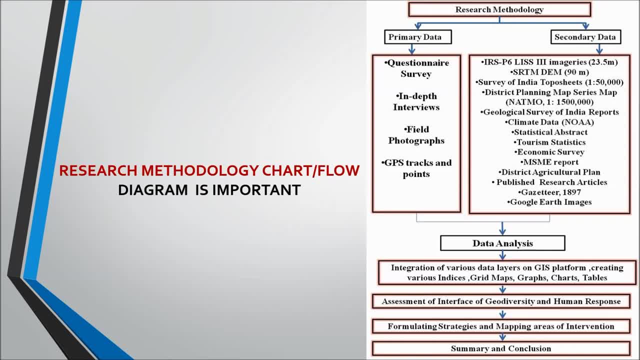 okay, so in written format of the report, this must come into the picture and then you can write it in the beginning of the chapter. so you can write it in the beginning of the chapter that what is your research methodology chart, just after your objectives, you must give your research methodology, because your objectives are going to be fulfilled by this. 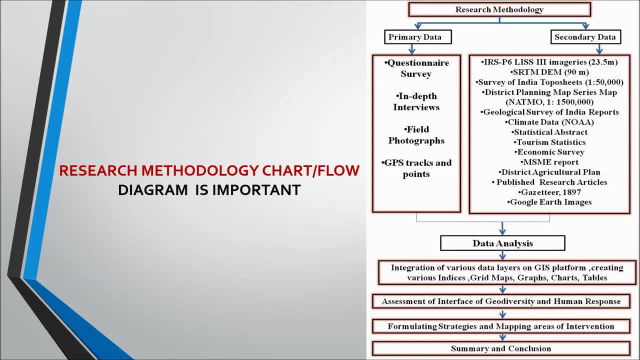 entire chart in this particular flow. so making such a chart gives a good impression to any reader. any uh tutor mentor would recommend you to make this kind of chart for a proper research based analysis and report writing. all right now, data tabulation and representation- the first major part of today's session. so how to tabulate? 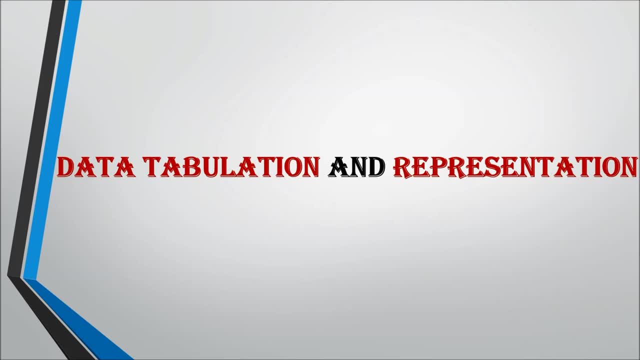 the data, what is the best method, what are the advantages and how to represent that. that's the important point of writing a report. finally, data collection is not enough. how to tabulate it, how to analyze it and then represent it is the main crux of the matter, because that is what is going. 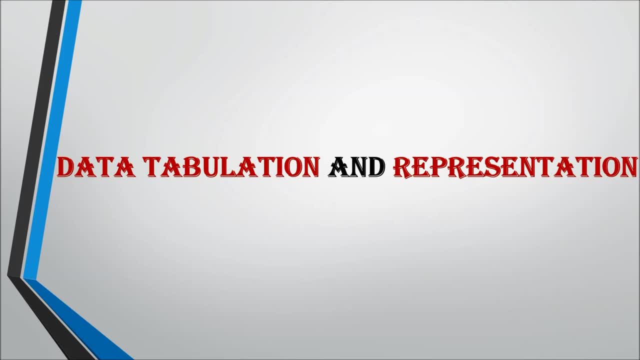 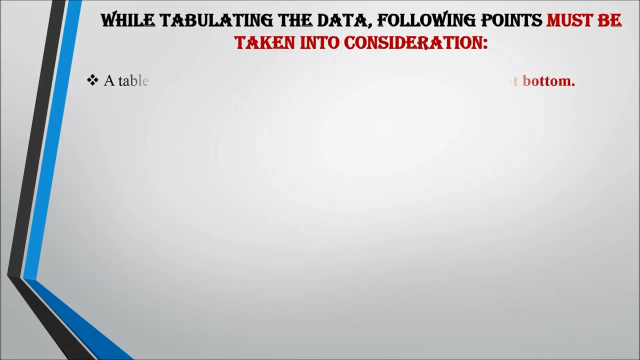 to matter at the end of the day. so remember, focus on the points that we are talking in this section of data tabulation and representation. so while tabulation, the data important point must be taken into consideration. first point: a table must have an appropriate title at the top and 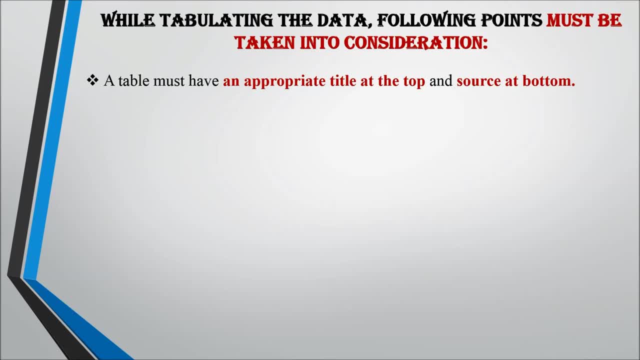 source at the bottom. okay, remember this point, for any table, of anywhere that you make a table cannot be titled less. so whatever you're making in the table you're providing, the information in the table must be having a particular title at the top in a bold form. 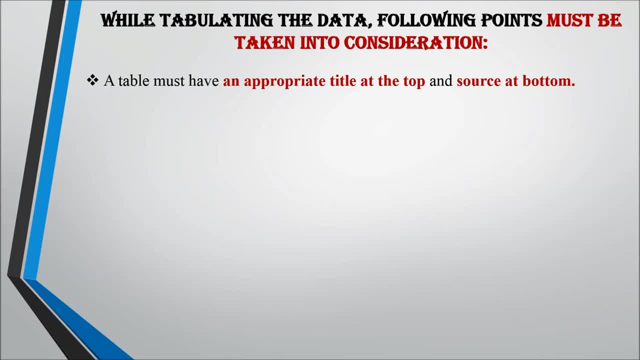 format or in a given format, that whatever is prescribed to you, but the format must remain uniform throughout. so remember, select a format and always post a title on the top and source at the bottom of the table. so if it is a primary survey based source, then simply write primary. 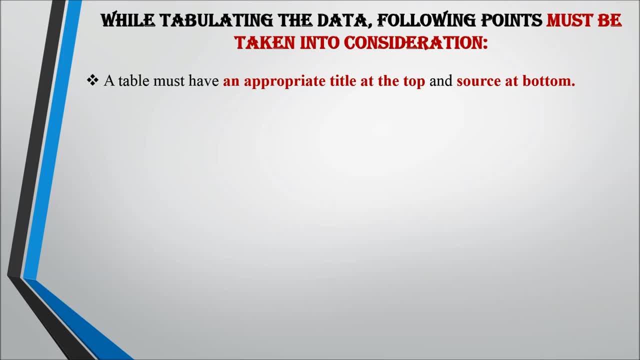 survey such and such here. primary survey comma. here don't write collected by the author, written by the author, done by the researcher. no, just write primary survey comma 2020 25. you want to write in whichever you have collected the data, so remember just a title at the top and 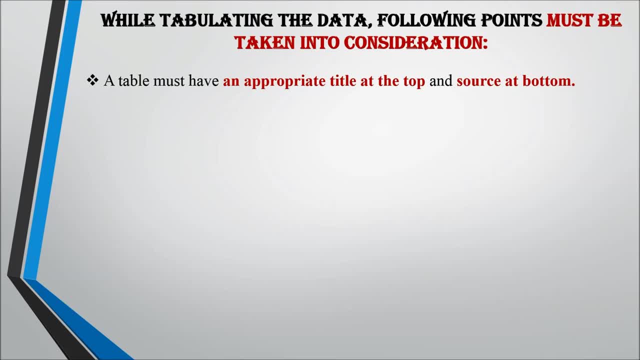 source at the bottom is the basic idea of the representation of a table. then further numbering is mandatory, so one table has to have a id of its own, isn't it? if you are having 30 tables- suppose you have made 30 tables from your questionnaire survey- then you can not have this distinguished. 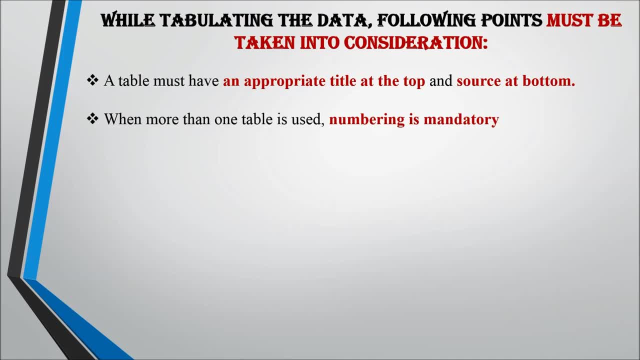 factor between all those tables without a number. so number is the identity. so suppose the table is in the first chapter, right? so first chapters, first table would be 1.1. that is the standard format. so for example, table 1.1 is for the first chapter, first table. 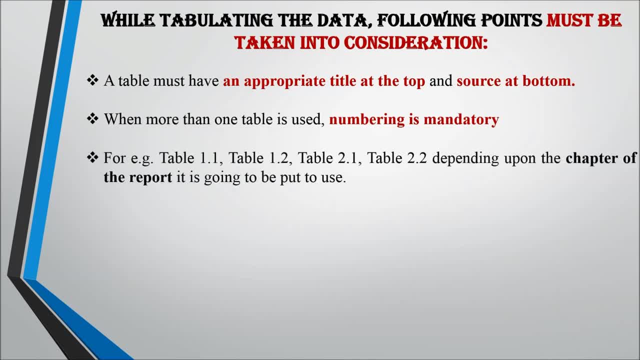 1.2 is for the first chapter, second table. similarly for second chapter, first table: 2.1. so remember that is a standard format of a report writing. in terms of table representation, always identify your table with a particular number, including the chapter number at the first and the second, chapter number at the second and the third and the. 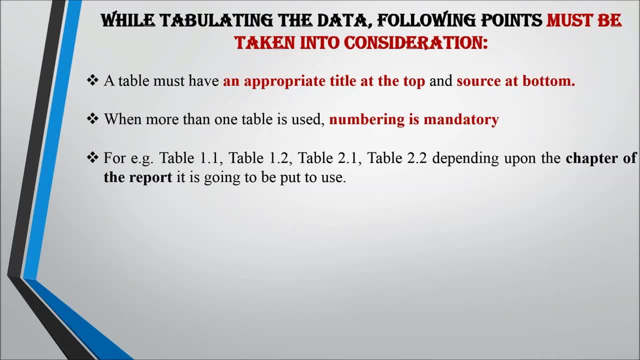 third and then with the table number. so table 1.1 means first table in the first chapter. okay, so remember that. then units of measurement and data representation must be clearly written. many times people miss this. they don't understand that. it's not a very much a good idea to leave. 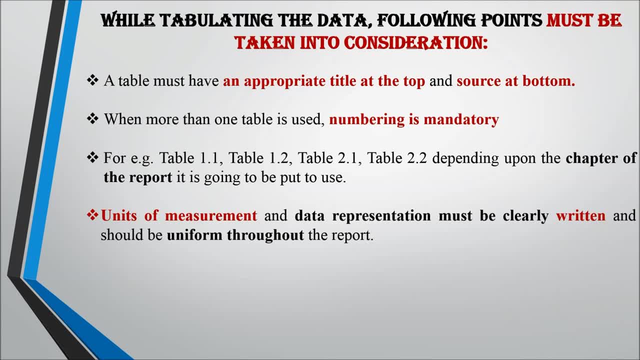 your data, just like, uh, any numbers, just in the form of numbers. units of measurements must be specified, because that will give a meaning to what you are trying to say through your data analysis, isn't it? so units of measurement is important and it should be throughout. it should be very uniform. 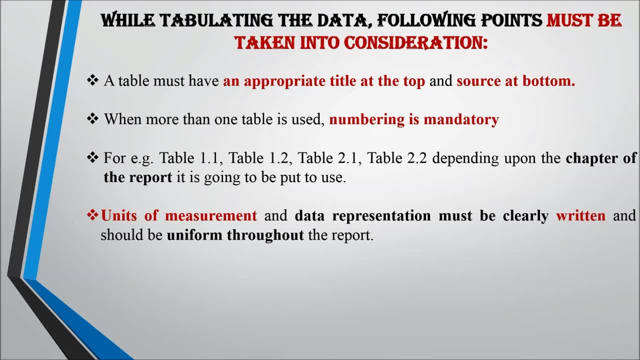 throughout. somewhere you have measured it into miles and somewhere into kilometers. if there is a particular distance, that's not fair. either use inch mile system or centimeter kilometer system. a standard format must be applied to units of measurement and representation of data. all right now in case of abbreviations that you use. if you're using an abbreviation, 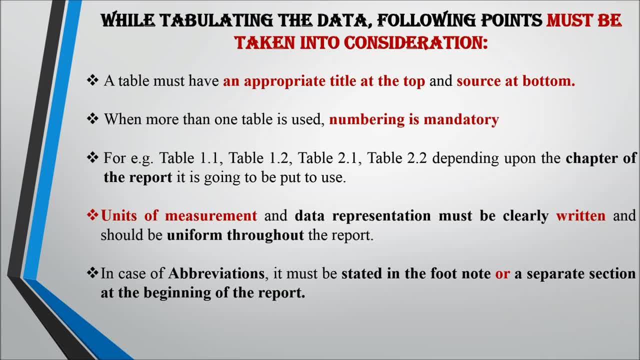 you must state it in a footnote section or at the beginning. you must add a page in which you can mention it, the entire abbreviations, acronyms, whatever you have used in this entire report further, so a person can refer to it. okay, and the best idea is to always quote that particular abbreviation in the paragraph. okay, 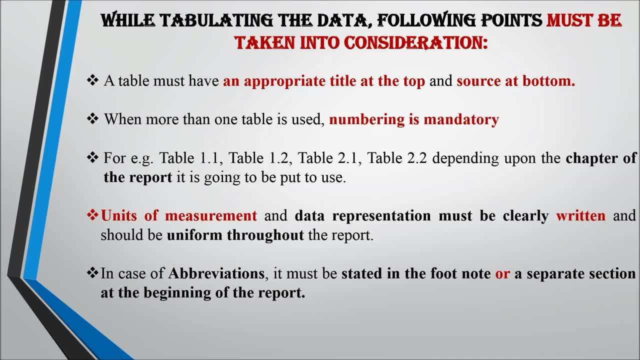 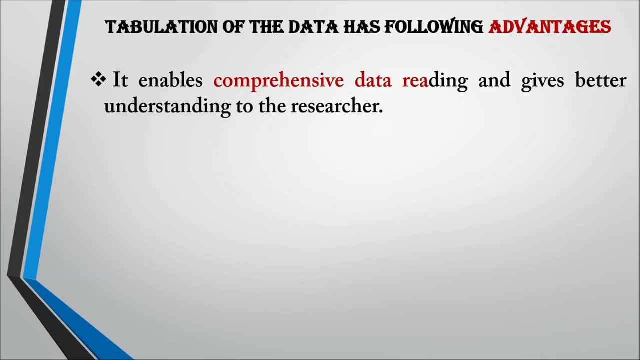 that you must state it. if, suppose, you are using usgs- united states geological survey- you must state it somewhere for the reader to understand what is usgs. all right now. it enables the advantages that it enables a comprehensive data reading for a researcher. if you have a, 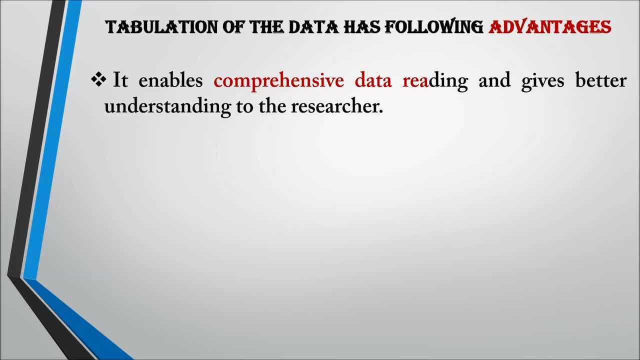 comprehensive approach. comprehensive approach basically means easy to comprehend, easy to understand. so if it is a comprehensive data reading method, that is only through good tabulation. so that is one advantage. then it fosters quick comparison between the variables. suppose i have to compare the variables. a good table would help me out to do it in a very fast manner. that's why 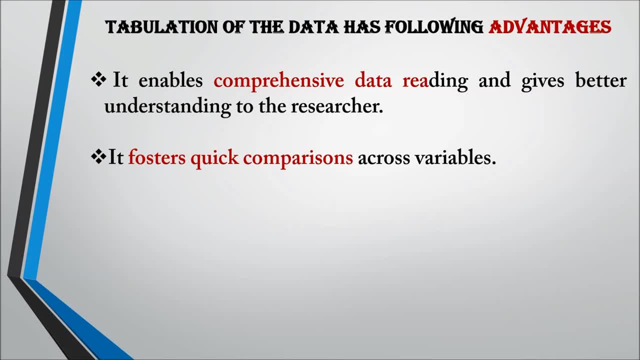 tabulation is important in a better manner. right, it helps to detect errors and omissions as well. you can find the missing numbers many times, isn't it through tables? now it precisely gives us the overall characteristics of the collected data. so good table, your representation is important. 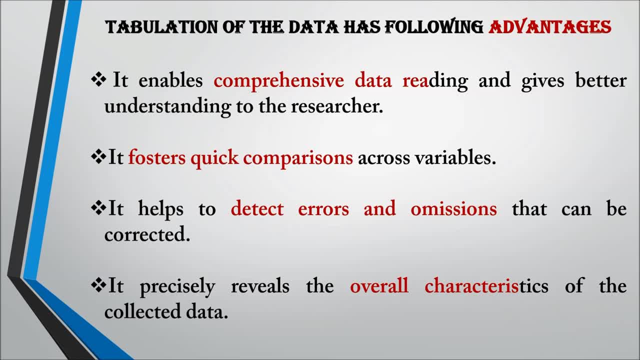 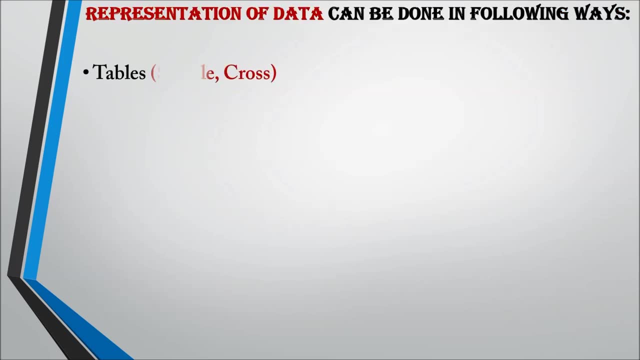 for this research part, the representation part, because this will give an reader the overall characteristics of the data collected and its analysis done. that's why tabulation plays a vital role in the analysis. and then further tables have to be simple or cross tables you can make for 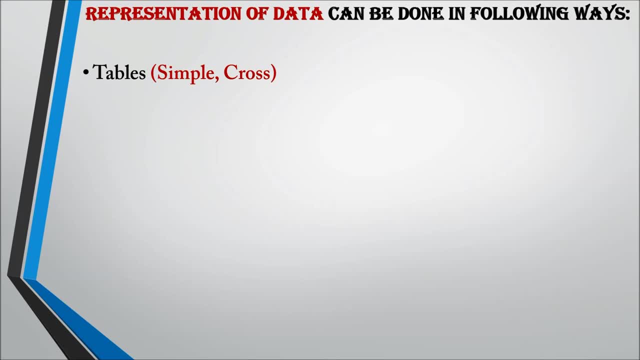 comparison right mapping is important part of writing a report. so mapping on the basis of gis software that we talked in the last session isn't it in the methods part? so use your gis software and always remember scale calculation through paste surveys if you have done in the field or 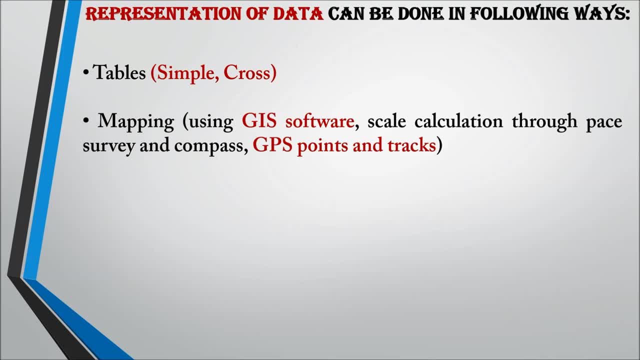 compass, gps points and tracks, it can be utilized to make a good representative map of the problem that you're stating. so the field report doesn't serve the purpose of a field report. remember, general map will only address the general problem, but field report is very specific so don't make generalizations of. 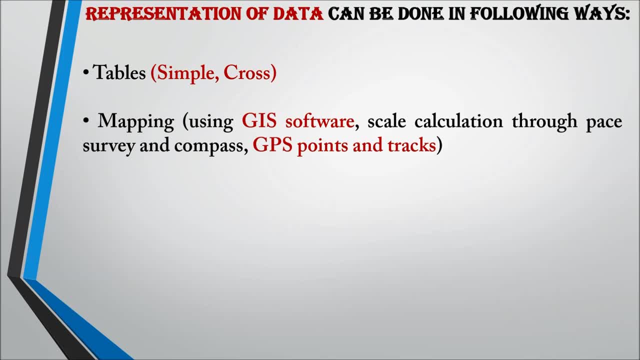 maps make it to the point, to the specific thing that you have done in the field. a map must be very specific, all right. now graphical representation becomes very much important: bar graphs, line graphs, star graphs, web graphs. you have so many options on the word format if you're 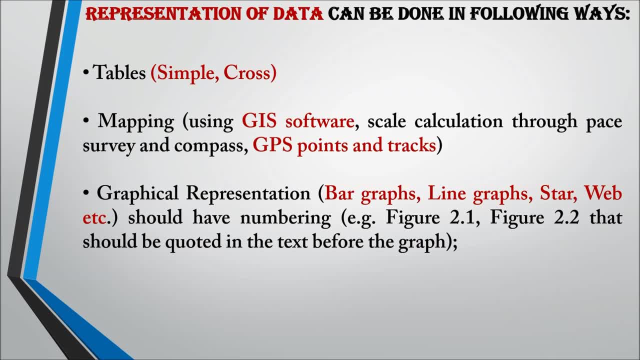 working, so you can use any particular format, so any particular word can be used for your files. you can use the data seven different version on the right. so you should have a good data on what your data is. all right, so you should have it numbered as well. again, the identity matters and graphical representations. 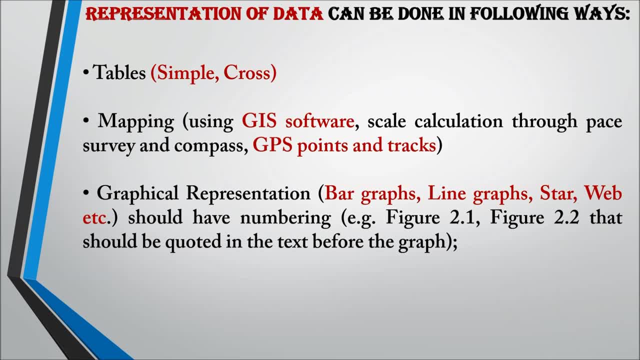 will be like. you have already discussed the tabular representation, so table 1.1. now it will be figure because it's a graph, graphical representations, so it can be figure 2.1, figure 2.2. certainly the identity has to be very clear of which chapter, which figure you are talking about. 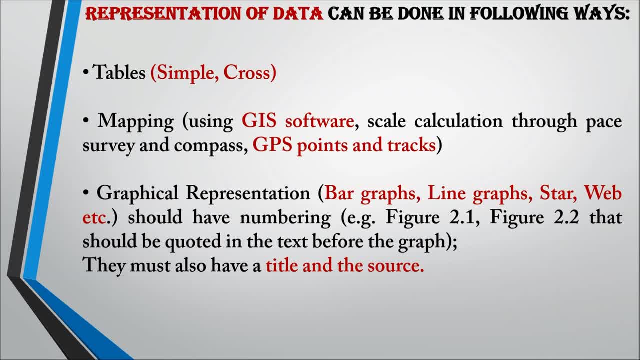 or it is a table, it must have a title and source. remember, do not forget to put the title and the source. if it is secondary data, secondary source. if it is primary data, write primary survey and the year. okay, don't write again. i'll repeat, don't write. collected by the researcher. 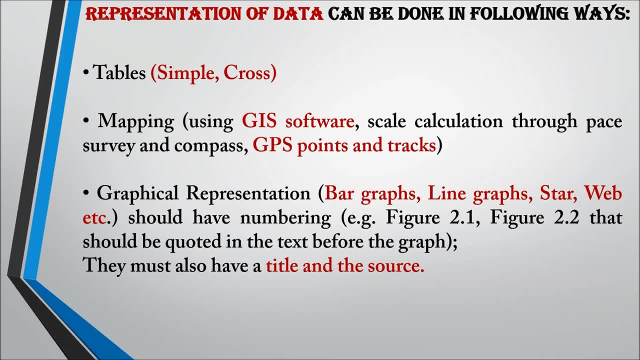 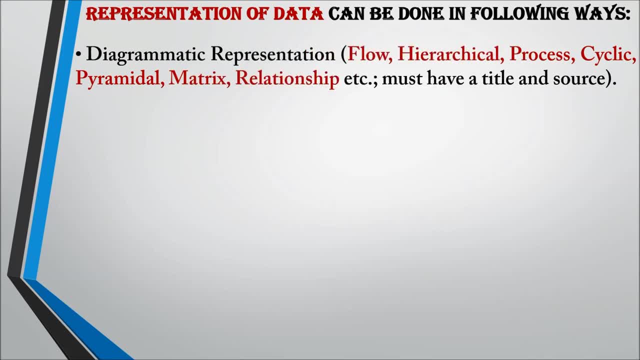 or analyzed by the author. don't write anything like that, just write primary survey. all right now diagrammatic representation, for example, flow diagram, hierarchy, process, cyclic pyramid matrix. many times of diagrams are available, but you must understand for what kind of representation you want a particular kind of flow. so you must be clear about the analysis, the data. so if you 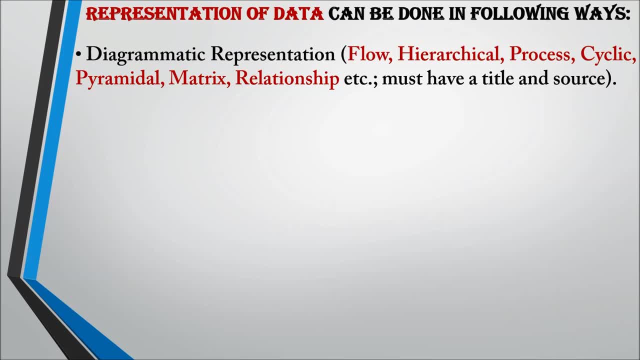 understand your data. you can pick and choose which kind of diagrammatic representation you want and, again, it must have a title and source. as we discussed, photographs cannot be just simple photographs. remember, you have to annotate your photographs well, if you are showing something in the photograph, it must be discussed in the 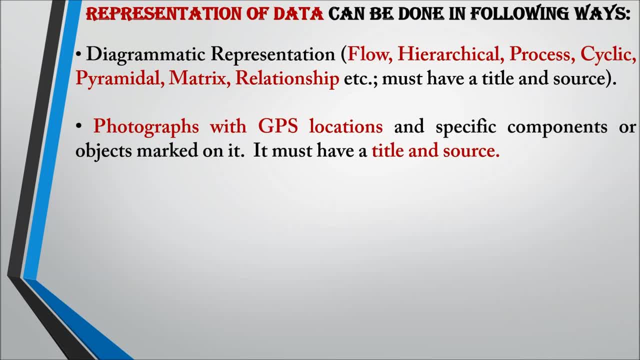 paragraph of the writing. as well as it must have a gps location or a google earth location, it must have a coordinate. okay, photographs cannot be left without any coordinates. so these days it's very easy: if you're carrying a gps you can put that gps location of the particular point of the 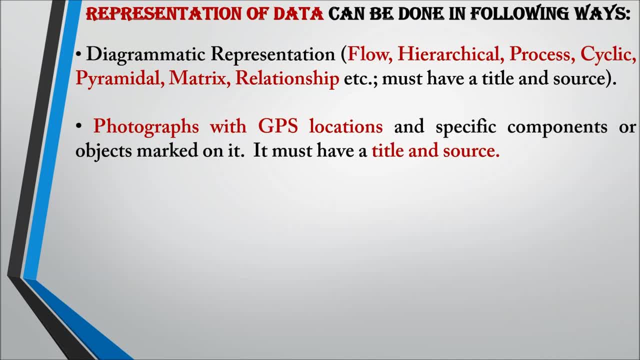 photograph, and you can, must you? you think that a photograph is something which a person is seeing it, but he is not able to guess the location. so you must specify a location and you must specify the location to him. okay, so that is the best way to actually geo tag your pictures. so 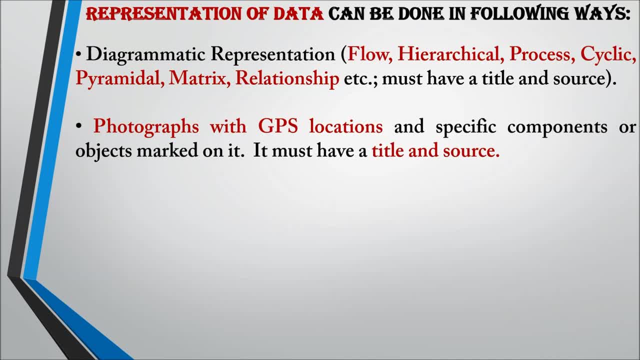 photographs must have gps locations or the coordinate points marked on it with the title and the source. obviously transcriptions of the recorded interview. so in the field, if you are talking about interviews to people, then those interviews must be transcribed. it must be written exactly the way it was said. suppose a person in the field says that we don't have any opportunity. 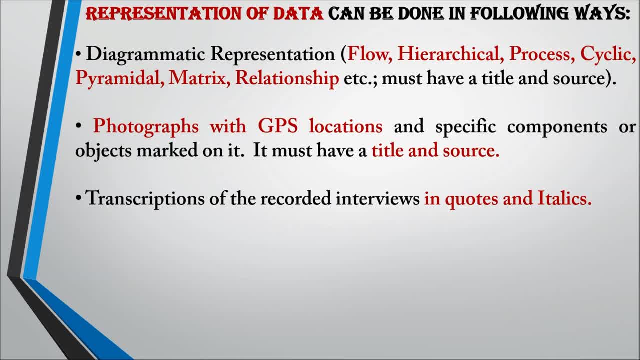 in the village to for further studies. so if you have recorded it, you must write in the same way, the same way that he has said that we that the respondent says that there is no opportunity for the higher studies in the village. so exactly, it should be written under quotes and in italics. so 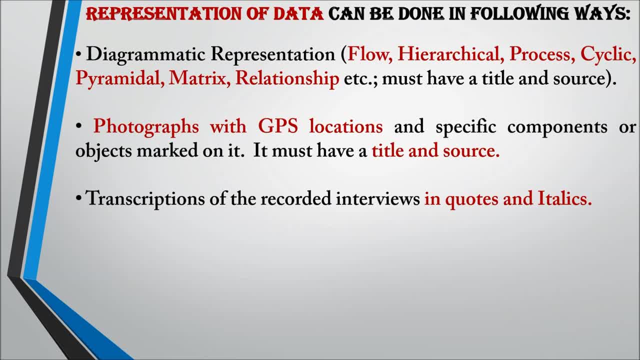 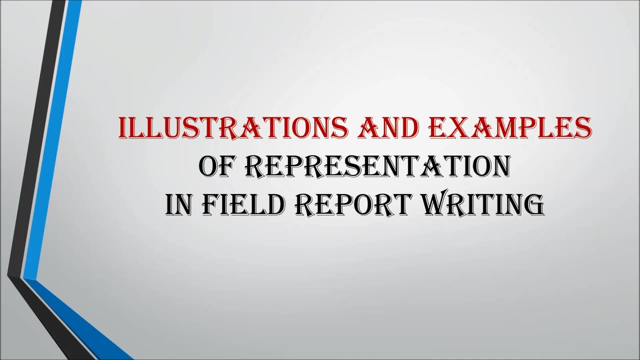 this is the way you transcribe your recorded interview right. sketches me made in the field can be scanned and put to use in the form of image. that is important. now i'll give you a certain illustrations and examples of representation that we have used in field work prior to this session. so i'll give an example now. look at this map. this map has a title: all the 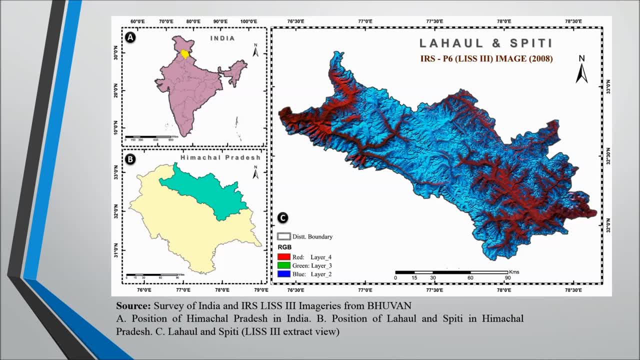 ingredients of a map and also it has a detailing of the sources. this map is based on gis analysis. so what kind of imagery was used? what was the source? what has been represented? so it is very clear to the reader that from this map was made, from what data source and what does it represent. 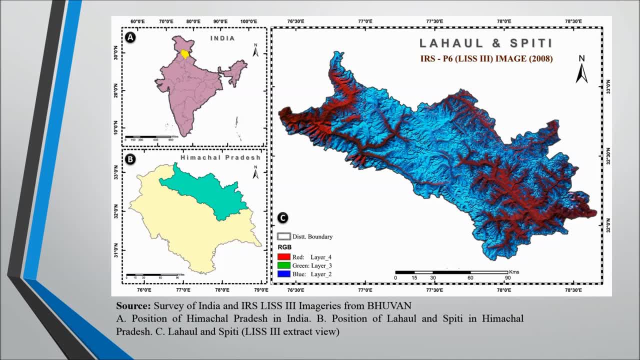 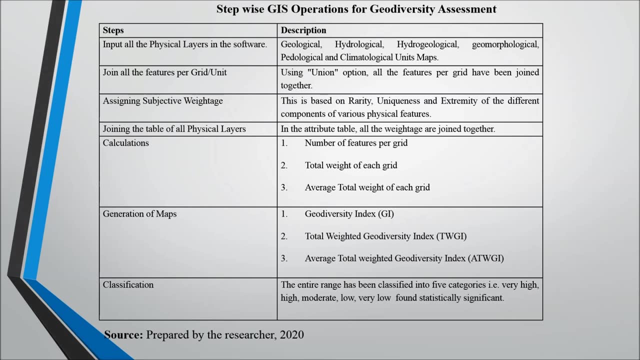 so map should be very clearly represented and it should be well quoted and title and as well as source must be there. okay, now any table. so this is another example of a table. but what is the title? stepwise gis operations for geodiversity assessment. so if you are making an analysis and assessment, 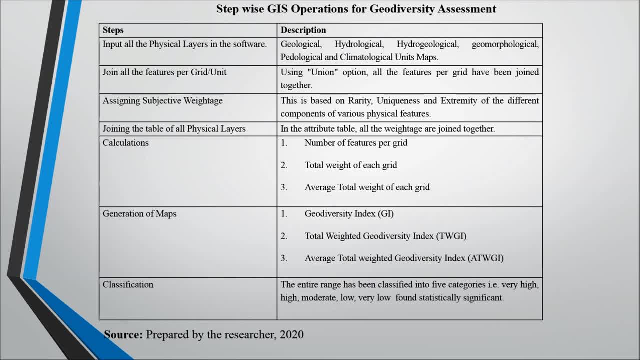 in which you are using a table, you must give a title and there must be a flow of all the steps that you have used in gis. so suppose you are using a gis operation to make a map, okay, so how will the reader understand? what are the steps? if i want to do the same mapping, how will i learn? 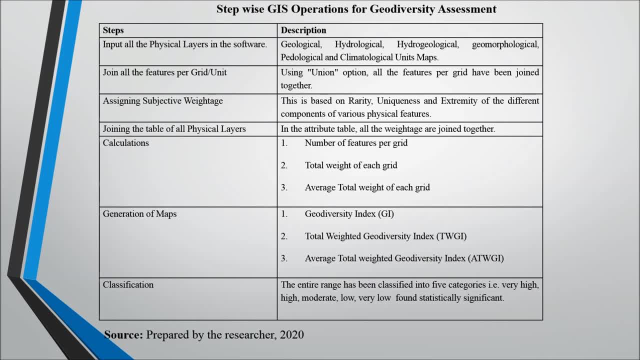 so make it easier for the reader by using the step method. always give the steps of gis operations when you are using it and always make the source as prepared by researcher in a given year. okay, so that is one of the important aspect. now, this is one of the ways you can represent a multivariate. 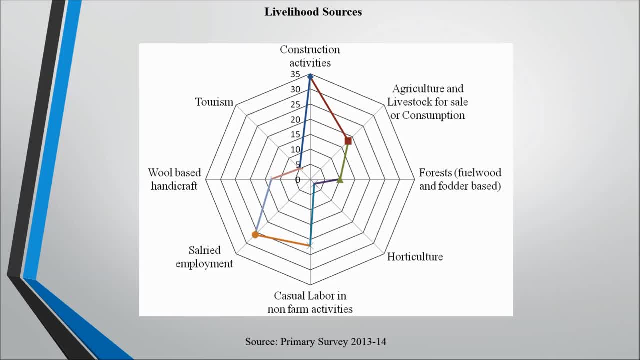 table okay, where you have lots of variations and you have many factors. so what you can do is you can create a web diagram, okay, and you can write it through primary source. in this it's very easy to identify what are the majority of factors that influences the title. so suppose here, livelihood is. 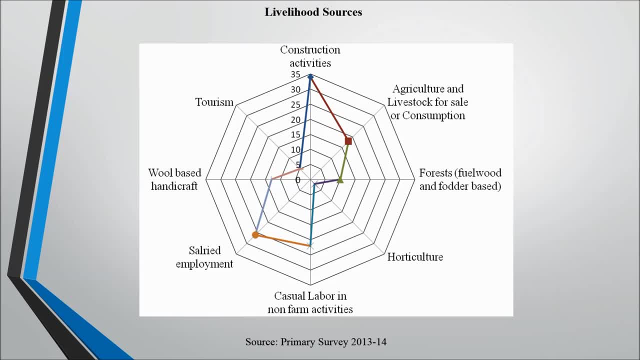 the title. so which are the more important factors in livelihood? so which axis is greater, construction activities, salaried employment? so these are the two major factors in the field area that is very clearly represented through this web diagram. so certain representations can be made in your field work as well. then these are certain types of pi diagrams. 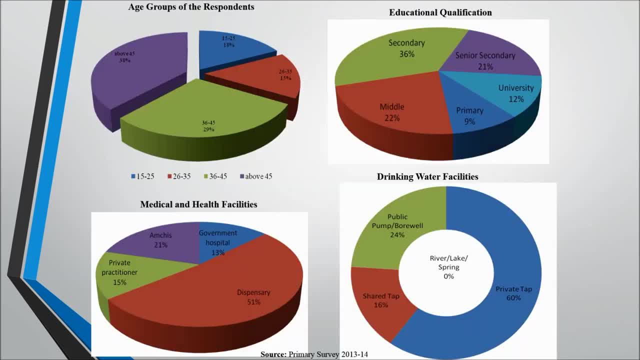 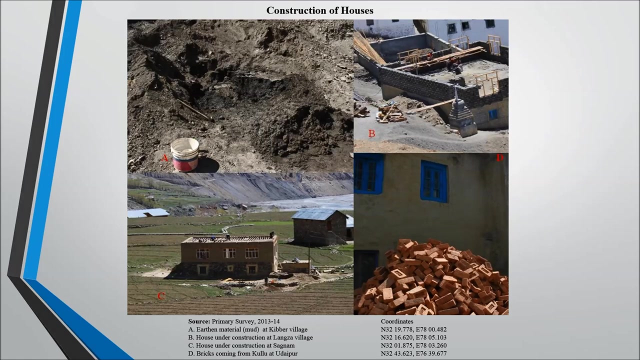 so age structure, educational qualification, medical health facilities, drinking water facilities. you can take any kind of pi and make it very clear with your title and source, specific and also representation of the y diagram. all right, now let's look at these photographs. so, as we discussed earlier, the title of the photograph, then mark the important identities of photograph if you're using. 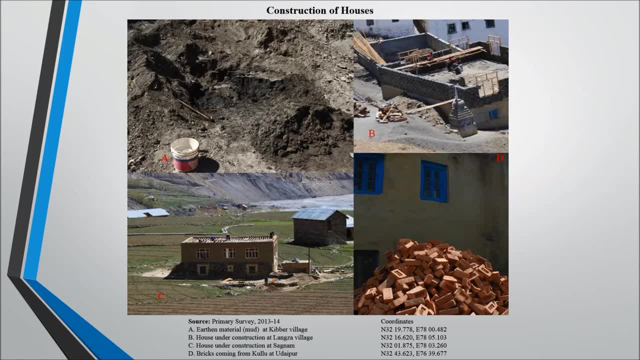 more than one photograph. so a, b, c, d and their coordinates have been mentioned. if you can see here, you can see the year in which they were taken. so title, source and coordinates must be there in your photographs of the field. you cannot use your random pictures in which you are standing. 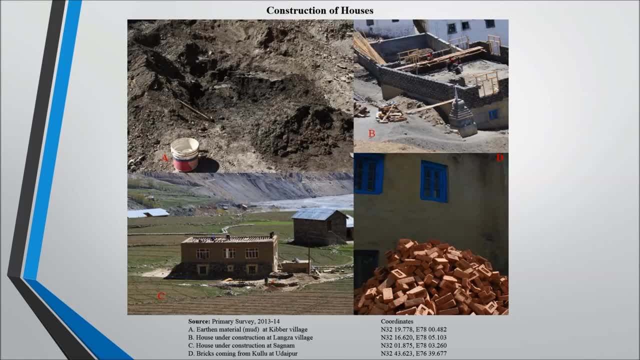 and clicking a selfie. please avoid using such pictures in the field. always remember: your pictures in the field must represent what you are trying to observe and identify. it should be fall in the context of your objectives, of your study. all right now, if you're using a google earth image, 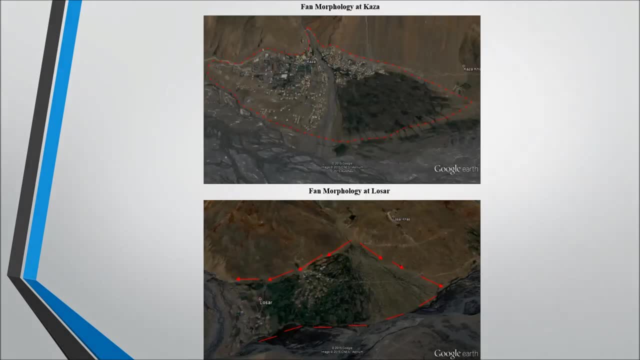 so it must have that bottom tagline of which year the google image was taken and also it should be marked, as you can see in the image, that just don't click a screenshot and paste it. remember, mark your images of the areas that you're representing specifically. as you can see, the images in this have been marked. 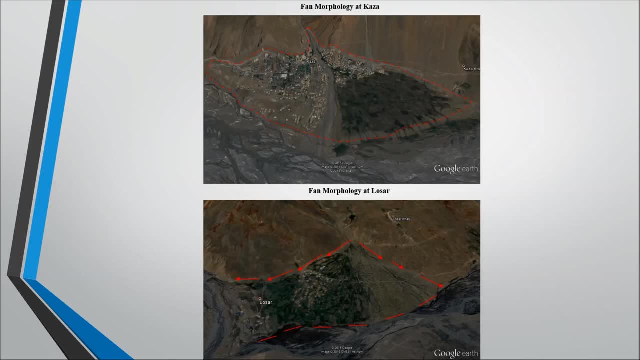 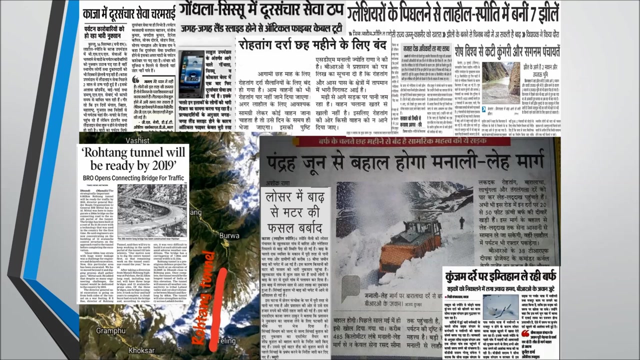 with red line, so mark it, then utilize for your reports. so that is the standard procedure of using a google earth map. right, you can use several field literature, for example. you can use new paper cuttings, but remember newspaper cuttings must have a date mentioned in their cuttings. so 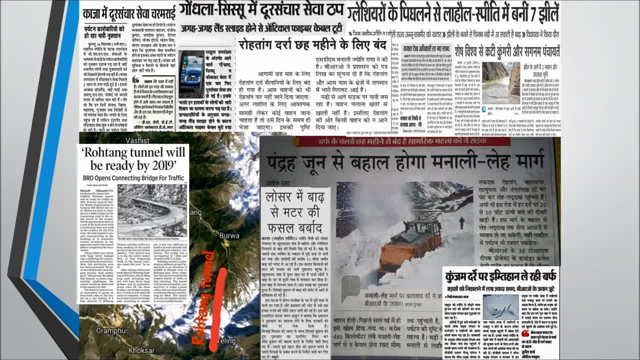 otherwise that's not fair to use it and it must have a title and source again. so title has to be what are you representing through the news and the source have to be which newspapers. if it is more than one newspaper, mark it and write one, two, three, four and the number of newspapers you have referred. 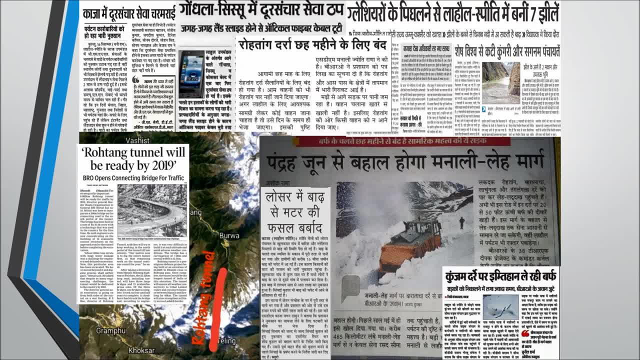 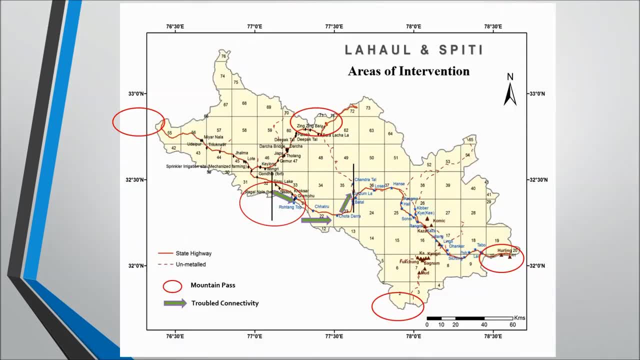 but the news items must have date mentioned in somewhere or the other. right now at the end you can also make an areas of intervention map. so if you have a study area map or sketch you can mark on that particular specific areas which you think that it has come up through your studies that those areas are needed attention. 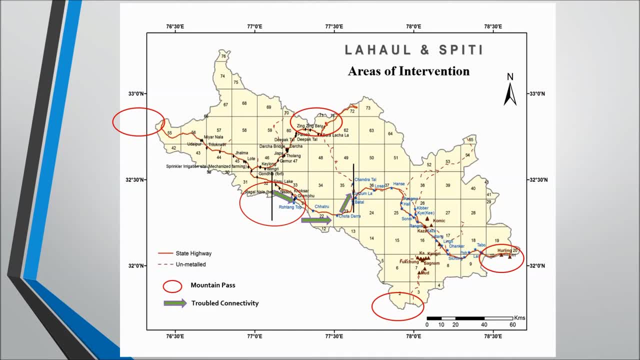 for any strategy, for any decision making, for improvement. so you can mark those areas and specify through that image in the last part of your summary of your writing of report. so end part, the conclusive part of your report, can have this strategies map or the areas of intervention map, because that would make sense to a reader that, okay, this person has done. 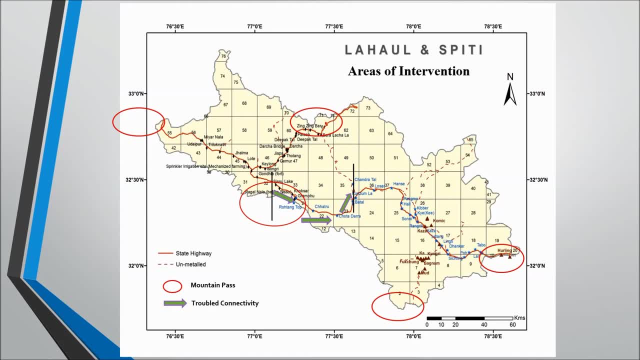 this research and now he's, she is providing this entire research into the framework of even making or formulating the strategies as suggested in the objectives part. so this is important to clearly mark out the particular areas of intervention or the areas of challenge or the areas where opportunities are there or threats are there. so anything but it has to be.